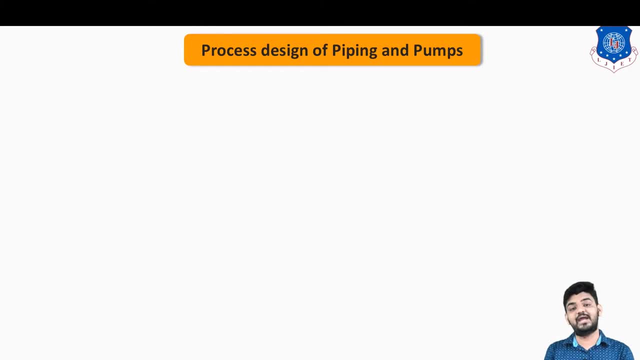 that chemical engineer can understand. how do we can design a chemical equipment that can be used for different unit operations? So in this video we are going to start our first chapter of this lecture. We are going to discuss the process design of piping and pumps. So basically, 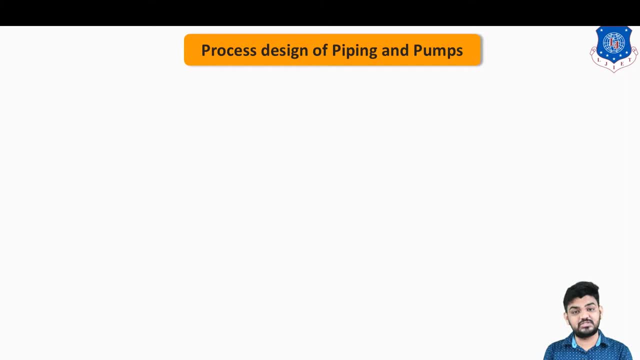 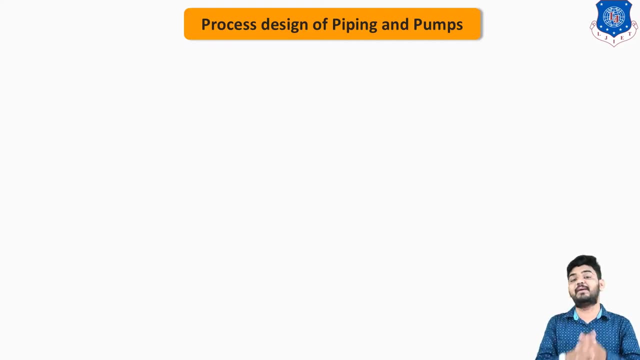 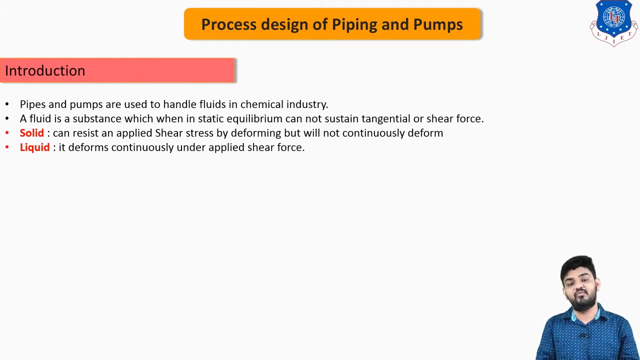 we are going to design devices that are being used to transfer fluids. So at this particular state, we must have to know what do we mean by the fluids, right? So in the, in the third semester and the subject of fluid flow operation, we have understand what do we mean by the fluids? 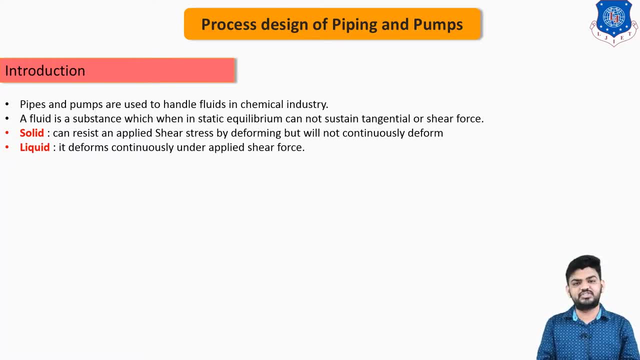 Basically, a substance can exist in a three form: solid gases and liquids. right, We distinguish all these three phases by their molecular forces or the internal arrangement of molecules inside the substance. right, But this definition to define different phases is very old. 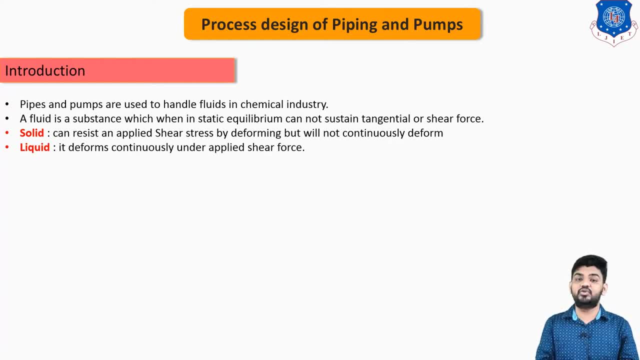 Now, in the seventh semester of the chemical engineer, you should be able to answer the how do we can define phase? or, specifically, how do we can define fluid? in a much more clear way, right? So here I have tried to explain you the definition for the fluid that a chemical 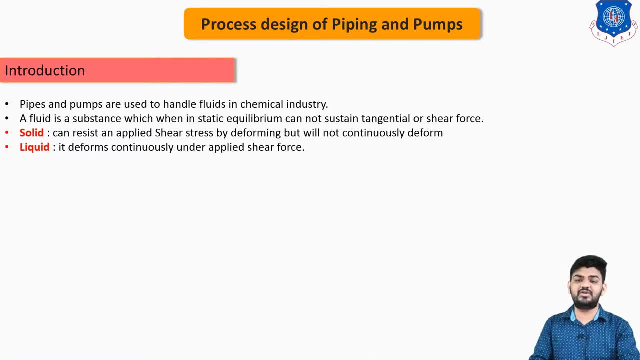 engineer need to be understand right. So, as you can see here on the screen, it goes like: a fluid is basically a substance which, when in a static equilibrium, cannot sustain tangential or shear force. That means whenever we try to apply shear force on a fluid, it will continue to deform. 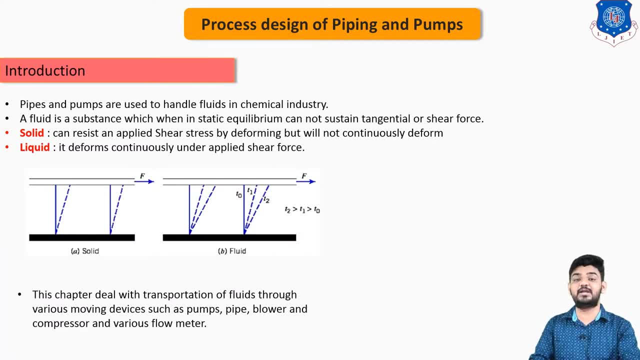 right. This definition can be easily understood by this particular image. As you can see here, this is this solid right. So whenever we try to implement external force in the form of tangential force such as this right So solid, will resist to deform itself. 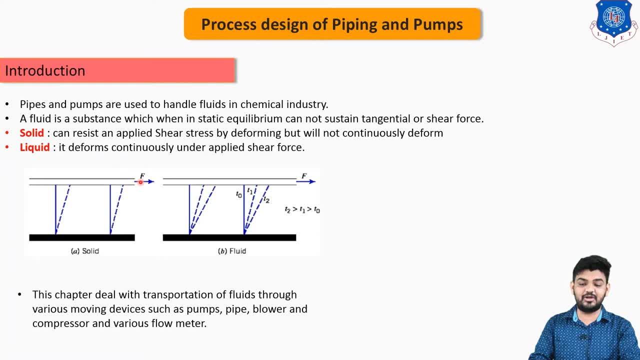 As you can see here, if I apply force in this particular direction. if this substance is in solid form, then it will resist its deformation, right. But in the same case with the liquid, as you can see here, if I try to apply shear force in this, 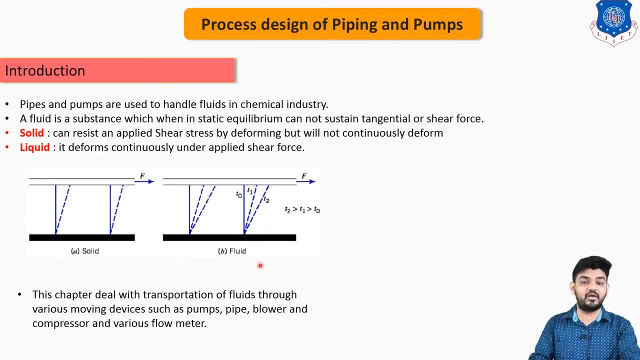 particular direction. and if this substance is liquid or a fluid, then it will continue to deform until this pressure or until this shear force is being removed, right? So basically now we can define solid as the. it can resist an applied shear stress by deforming, but it will not continue. 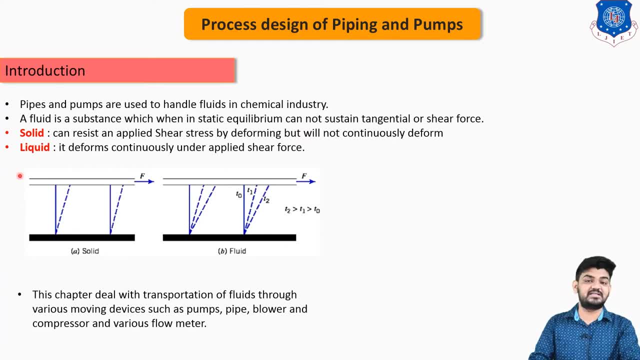 to deform right. So, as we have seen here, it can resist its deformation right. So, as we have seen here, this solid substance do not continue to deform right. The perfect example is the erasor. If you apply some sort of shear stress on the upper surface of the erasor, 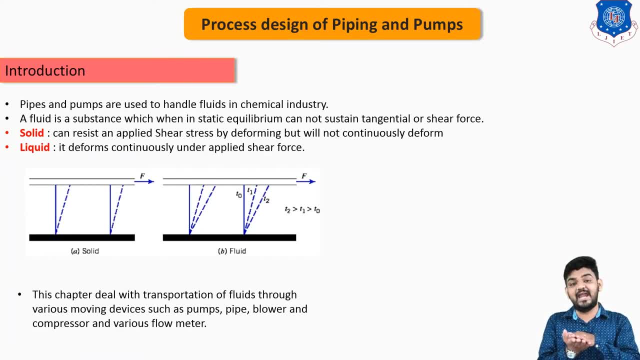 that will try to deform right, But at the end it will not deform continuously. On the another hand, if we apply the shear force to the fluids, they will continue to deform. right Example is if water fall on the surface, it will continue. 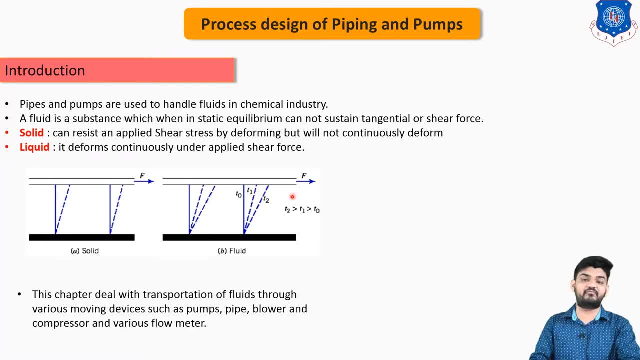 to deform until the shear force is being removed from the top side. right. So this is how we can define solid and fluids. So this is the perfect definition to explain the fluids, or we can say differentiate between solids and fluids. right? So basically, solid, do not continue to deform. 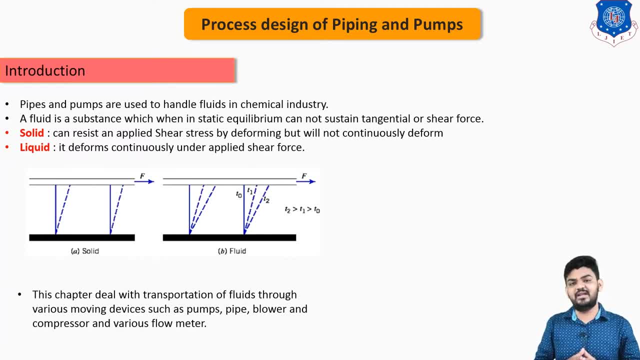 when their shear force is being applied on them, While liquid, as you can see here, liquid is continue to deform as under the applied shear force. So whenever we apply shear force on liquid, they will continue to deform right. So up till now we have understand. what do we mean? 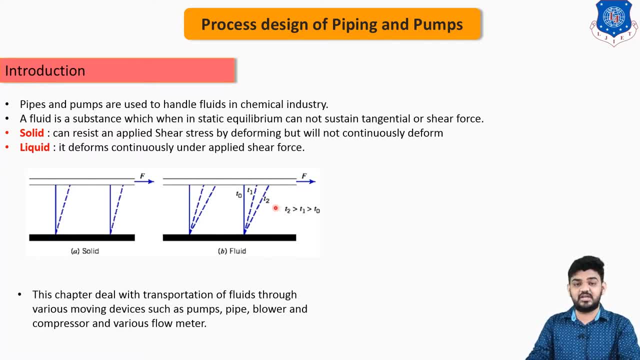 by the fluid. Now, in upcoming section, we are going to discuss how do we can transport this particular fluid right? So, basically, this chapter is dealing with the transportation of the fluid through various moving devices right. This devices can be pumps, pipes, they can be blowers, fans, compressor, and in the end we are going to discuss 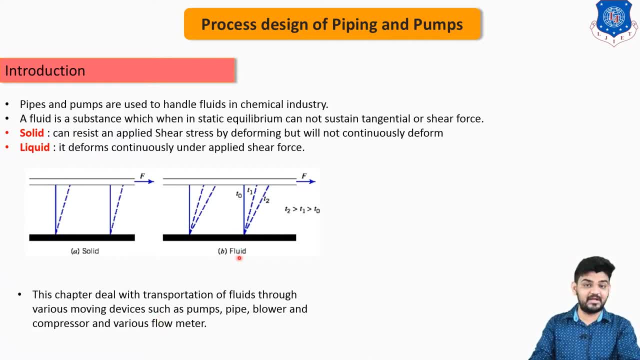 about the different flow meters. So this particular chapter is very important for the exam point of view and in this chapter we are going to require a deep understanding of the fluid flow operations. So now, after discussing or after introducing this chapter, let us move. 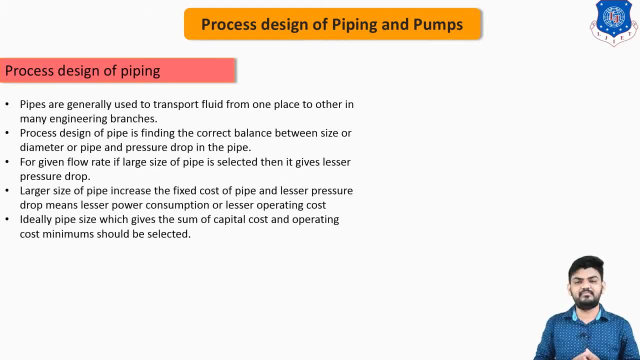 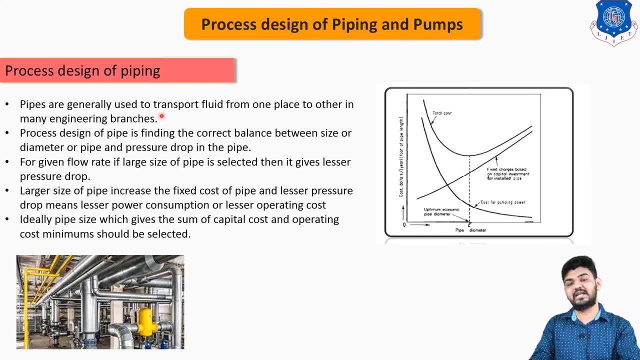 to the process design of pipes. That means: how do we can design the fluid flow meters? So let us move to the process design of pipes. So, as you can see here, pipes are basically generally used to transport fluid from one place to another place, right, As you can see here in the image, that different pipes are being used. 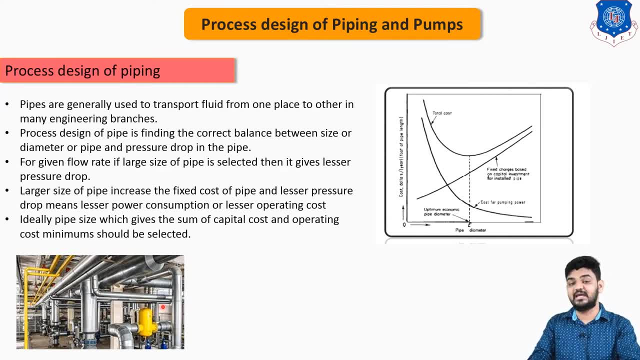 to transport fluid from one place to another place in the industry, right? So process designing of the pipe is basically nothing but finding the correct balance between size of the pipe and pressure drop inside the pipes. So basically, we have to design pipe in a such a way that it is the 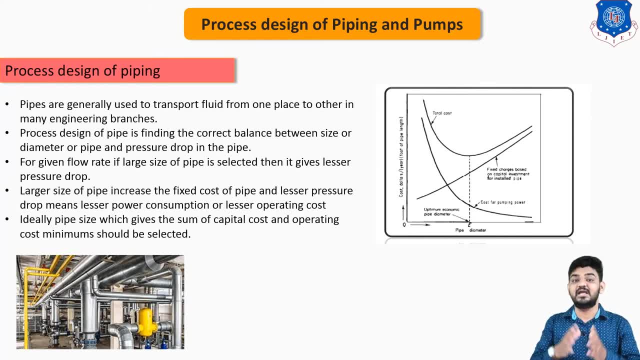 perfect balance of size of pipe. That means the diameter of pipe and pressure drop of the pipe, As both the things are completely opposite, right? If we increases the size of pipe, that is, if we increase the diameter of our pipe, then it will give lower pressure drop, Which means we can easily 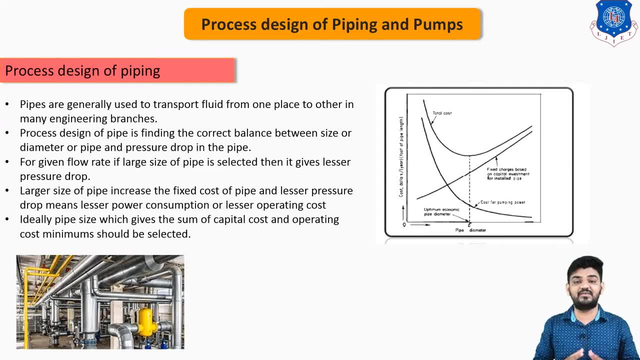 transport our fluid from one place to another place in the industry, right. So this is the process: from one place to another place with the help of large diameter of the pipe, But, on the another hand, if we continue to increase diameter of our pipe, which ultimately affect the fixed cost of pipe. 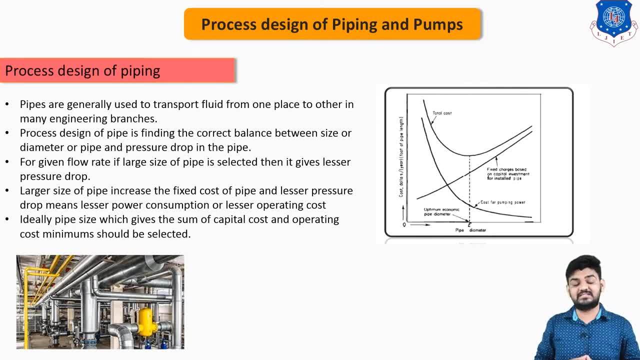 right, As larger size of, as larger diameter size pipe are very costly than this lower one, right? So as a chemical engineer here we have to define the perfect balance between size of pipe and pressure drop inside the pipe, right? So, as you can see here in this, 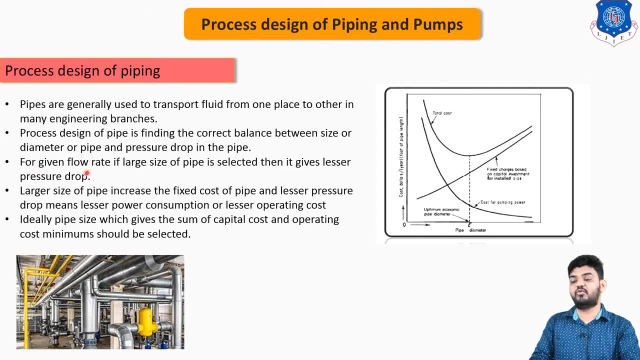 So, as you can see here, for a given flow rate, if we select larger size of the pipe then it will give lesser pressure drop, as I have already discussed right. So lesser pressure drop means we can easily transport our fluid from one place to another place. That means the pumping cost of our fluid. 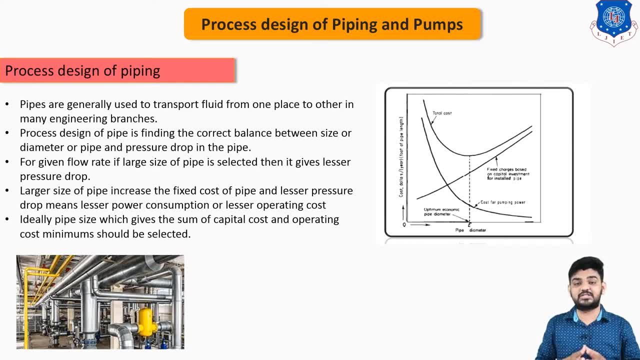 is very low, Which means the operating cost of our fluid is very low. So we can easily transport our fluid from one place to another place. That means the pumping cost is very low. But on the another hand, as you can see here, larger size of the pipe increases the fixed cost of pipe and lesser pressure drop. 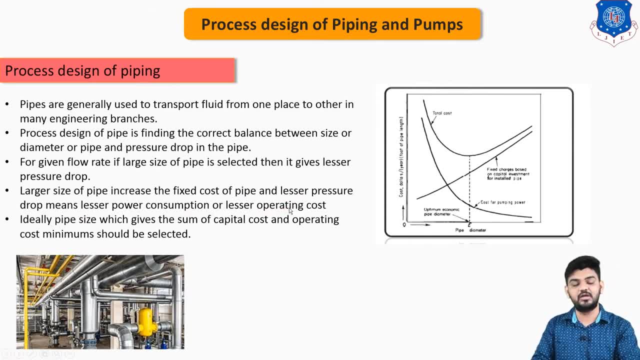 means lower power consumption or lesser operating cost, right? So, basically, if we select larger size of the pipe, it will decrease operating cost, but it will increase its fixed cost or capital cost, right? So we have to find the perfect balance between these two quantities, That is, operating cost, and. 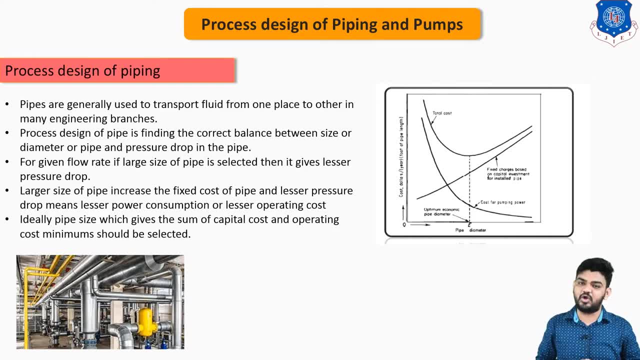 fixed cost of the pipe based on the diameter of selected pipe. So, as you can see here in this particular image, as if we continue to increase our diameter of pipe, the pressure drop through the pipe continue to decrease. as you can see here, this particular line shows the pressure drop. 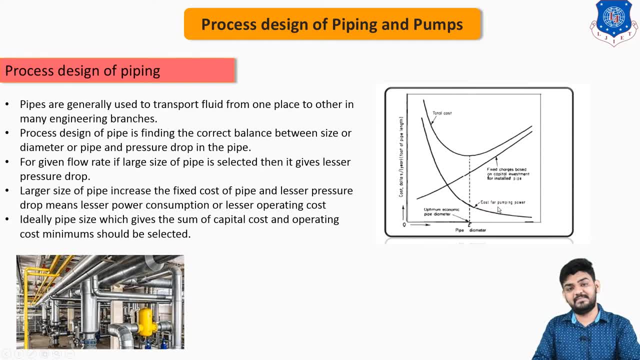 versus diameter of pipe And similar way, if we continue to increase our diameter then it will increase the fixed cost or the capital cost of our pipe. So ideally we should select a point where our total cost, that is, operating cost and the fixed cost, is minimum. 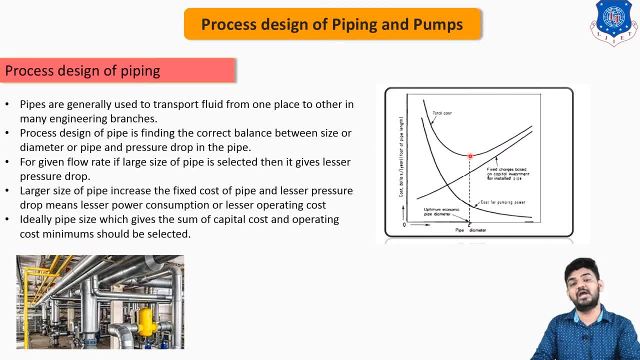 So this particular point can be considered as the optimum diameter point, right? So, as you can see here, ideally pipe size which gives the sum of capital cost and operating cost minimum should be selected. So while designing our pipes, we have to keep two things in a mind. that first one is the size of 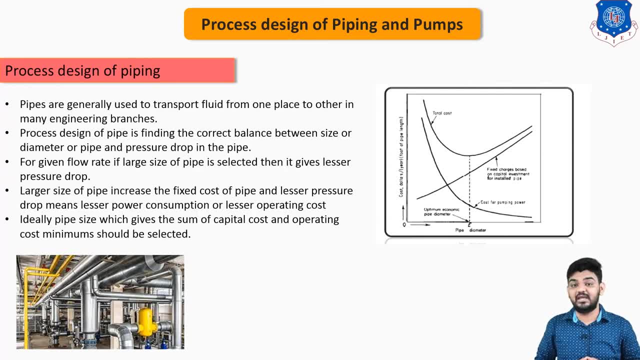 pipe, that is nothing but your diameter, and another one is the pressure drop right. So we have to find perfect balance between two, these two quantities right. So now, as we have already discussed, what do we mean by the optimum diameter? let us understand how. 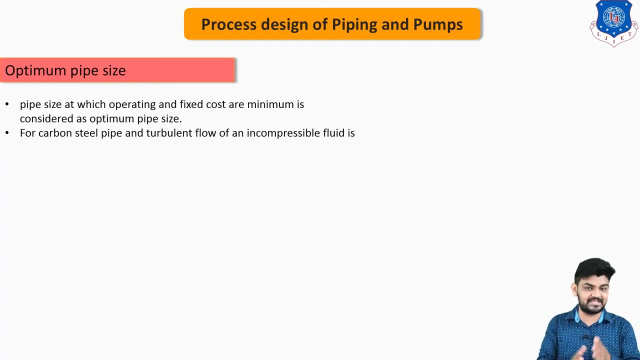 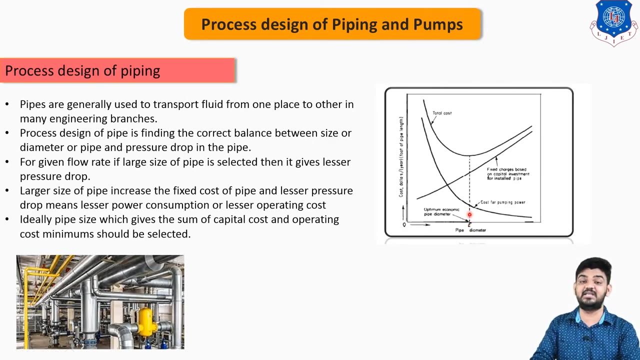 do? we can find this optimum diameter or we can say optimum size of pipe. As you can see here, pipe size, at which operating cost and fixed cost are minimum, is considered as the optimum diameter. So in a previous slide you can see here this particular point is being considered as the. 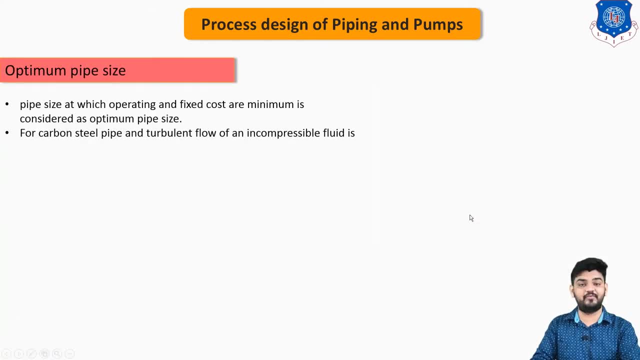 optimum diameter and we have to define or we have to find this optimum diameter. So for the carbon, steel and turbulent flow with incompressible fluid, we can easily define this optimum diameter as d of t, that is, the optimum diameter is equal to 293 into mass flow rate, raised to 0.53, which is multiplied by density of our fluid, which has 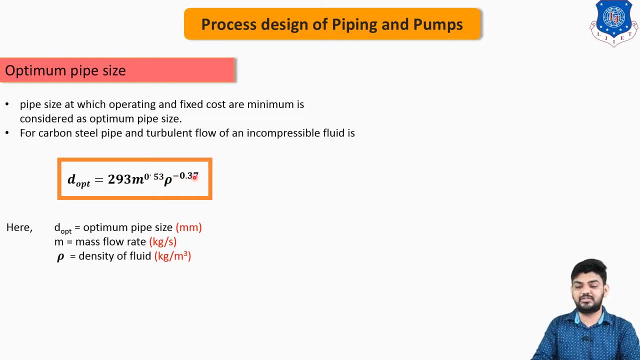 raised to minus 0.37.. So this particular formula is again very important in order to calculate the optimum diameter of our pipe. As there are so many questions that has been asked in GTU exam to find the optimum diameter of pipe. even in some cases this question has also be asked in. 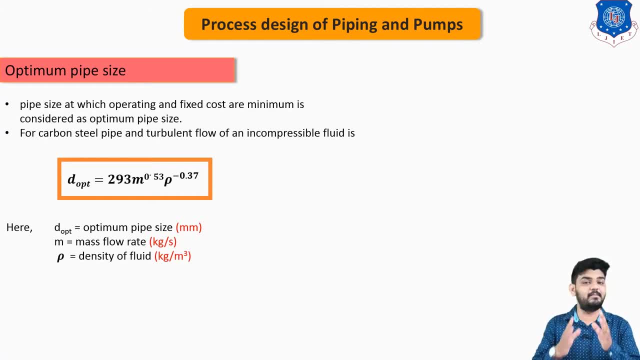 the gate exam as well. So for that purpose, you need to remember only this simple formula: that the optimum is equal to 293 into mass flow rate raised to 0.53, into density raised to minus 0.37.. So, as you can see, here, the here, the optimum is nothing but your optimum size of pipe. 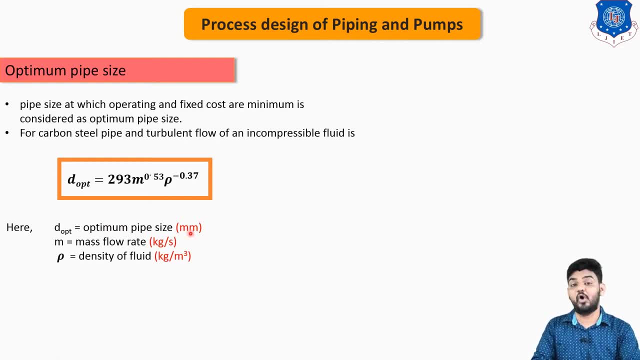 which is in the millimeter right. So here you have to always remember that this unit of d optimum is mm right. then we have m, which means mass flow rate, and unit of this is equal to kg per second right. and then, lastly, we have density, which has unit of kg. 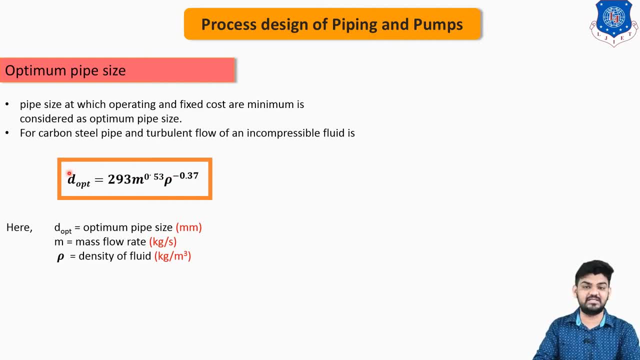 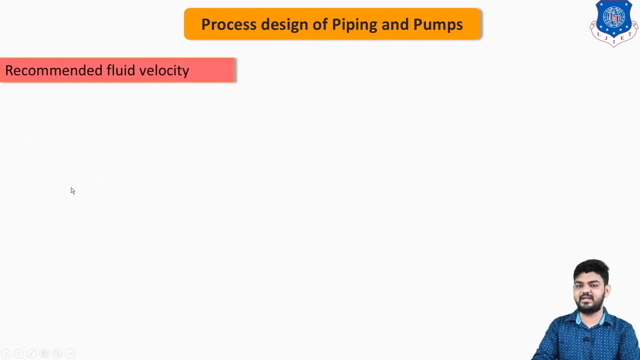 per meter cube. So if we implement these three things, we will be easily calculating the optimum diameter for our pipes. Now, after discussing this optimum diameter, let us understand the recommended fluid velocity. So, as you can see here on the screen, that recommended fluid velocity can be used to. 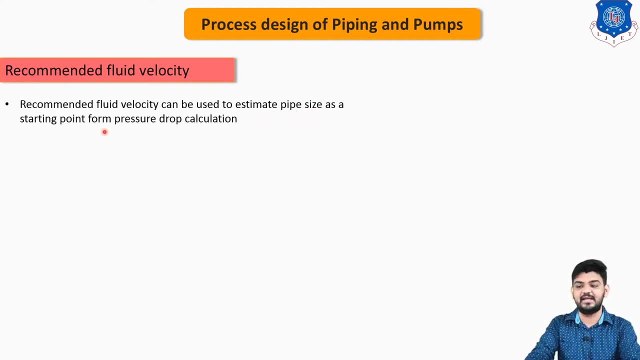 estimate the pipe size, or we can say pipe diameter, as a starting point for the pressure drop calculation. So whenever we have to design our piping system, we have to always calculate the pressure drop inside that pipe. So in order to calculate this pressure drop, we have to. 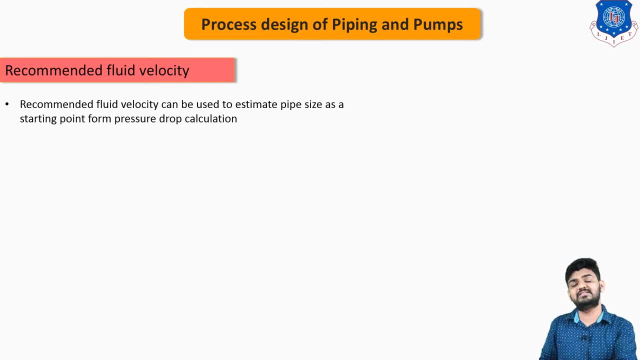 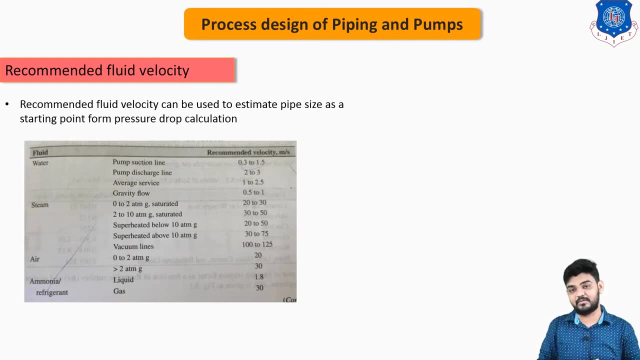 initially assume some velocity. So here are the some recommended velocity that can be considered for the starting point of the pressure drop. So here are the some recommended velocity that can be considered for the starting point of the evaluation of pressure drop inside the pipe. 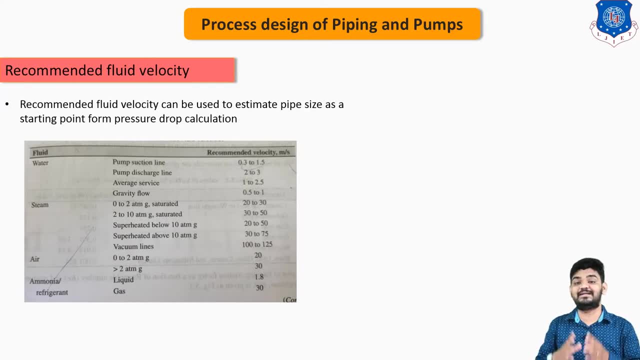 and based on this velocity, we need to calculate diameter of our pipe, and that thing we will understand while we are solving this sums based on this pipe system. As you can see here, if our fluid is water which is being used for the pumping suction line, then it has to be in the range of 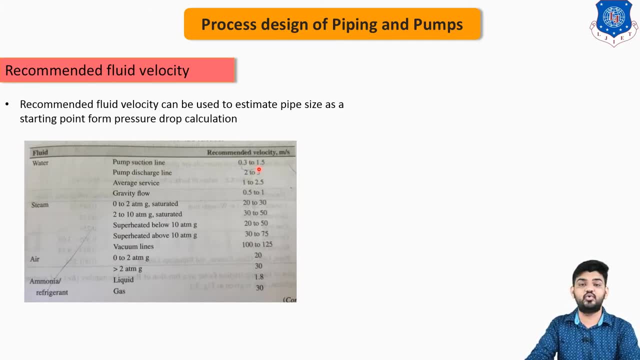 then its velocity should be in the range of 0.3 to 1.5 meter per second and same value for the discharge line. the velocity increases from 2 to 3 meter per second, And similarly the stream has the velocity of 20 to 30 meter per second. If we are using air for some purposes, then it has to be. 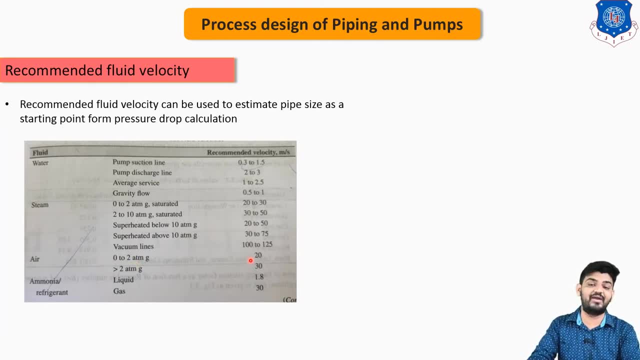 followed this velocity of 20 meter per cent right. So these all are the recommended velocity for different fluid that we need to understand our we have to use for our calculation purpose And for the exam point of view. we always need to calculate right: 20 meter per second form our equation. So this would be 20 meter per second, then if the distribution can be improved for higher. Но there is a following tension, and that is equal to 1 meter to 30 meter per second. what that value, which will be the parameter for we can check this? notice that if시면 temperature. 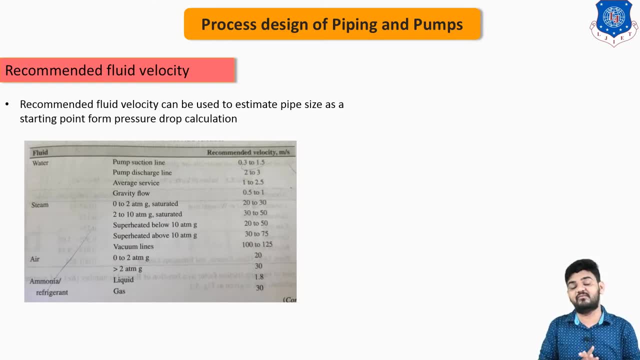 of you. we always need to remember what are the recommended fluid velocity so that we can initialize our calculation and that part we will cover when we solve some based on this particular thing right So now, after discussing this fluid velocity, let us continue our discussion on the pressure. 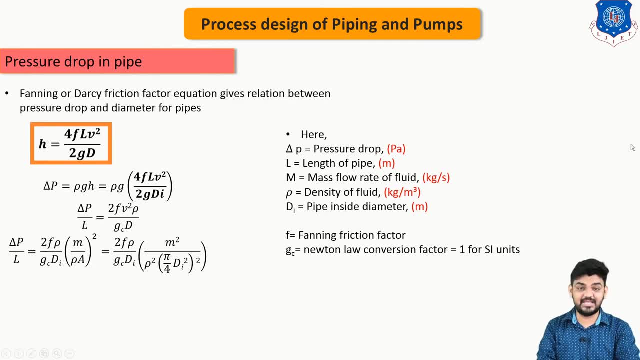 drop calculation. So basically this is one of the main step in the determination or designing the piping system. So as you can see here, basically pressure drop inside the pipe can be determined by the fanning or the Darcy friction factor. as this fanning or the Darcy friction factor 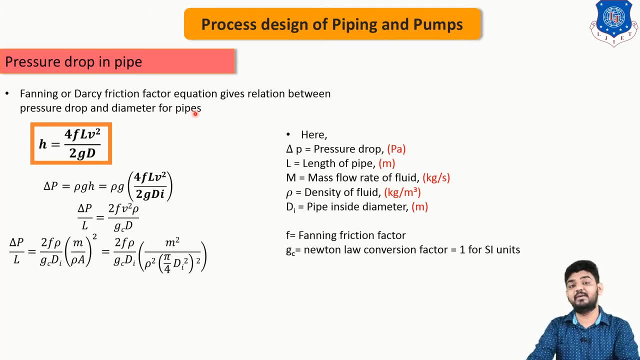 has the relation between pressure drop and the diameter of pipe. So let us just recall, in the fluid flow operation we have understand the relation between head, the relation between head loss and the fanning friction factor, as H is equal to 0. So this is equal to 4 f L V square by 2 g V right. this equation we have understand in. 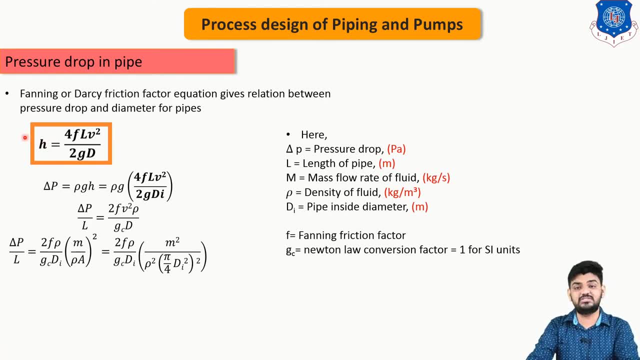 the fluid flow operation, and again we are going to use this particular equation for the piping system here in this PED subject as well. So this H basically stands for height. So here you can see that from this particular height if we have to calculate our pressure. 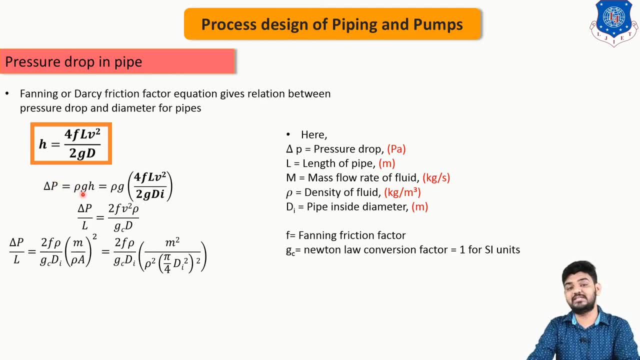 drop, then delta P is equal to rho 0.. So here you can see that from this particular height, if we have to calculate our pressure drop, then delta P is equal to rho g H. and now here this H will be replaced by this equation, that is, 4 f L V square by 2 g V. 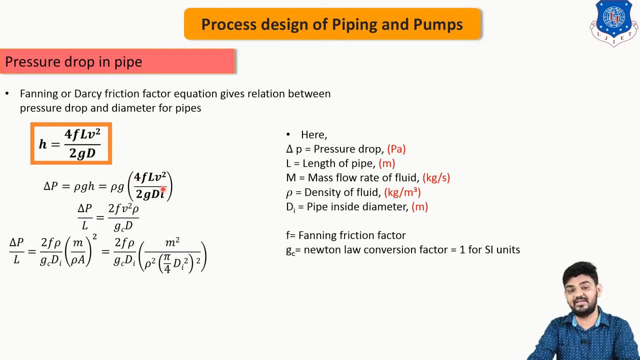 So, as you can see, here I have replaced this particular equation, in which I have replaced D, with the D I, which is nothing but your internal diameter of pipe. Based on this, we are going to calculate our pressure drop right. So if I take this length of our pipe to the left hand side, then we will have delta P by 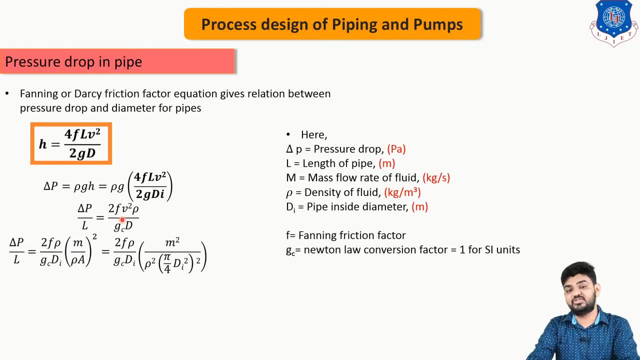 L, Which is equal to 2 f P square rho divided by g C into D. Now here, this g C is nothing but g by G. that is Newton law conversion. right, That is Newton law conversion, and which is equal to 1 when we are using SI units. 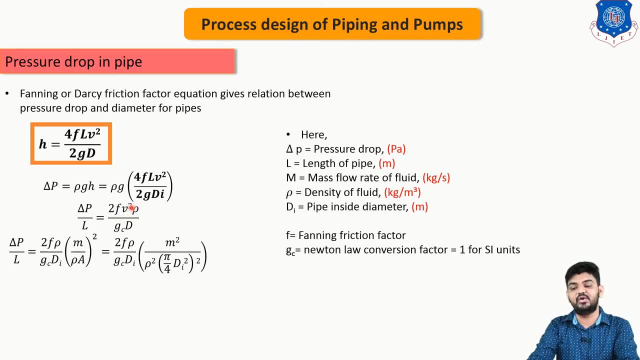 So, as you can see here, now we are going to replace our V with M by rho A. that is nothing but your continuity equation, which is says that mass flow rate is equal to 0. So if I make velocity as a subject, then we will have: velocity is equal to mass flow rate. 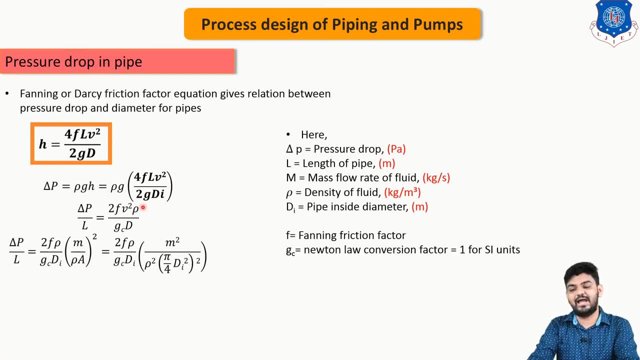 divided by rho into its area. So now I have replaced velocity with M by rho A and now I have to square entire bracket. So if I solve this particular bracket then I will have 2 f rho divided by g C into D I. So I have to square entire bracket. M square, rho square and area of pipe can be evaluated. 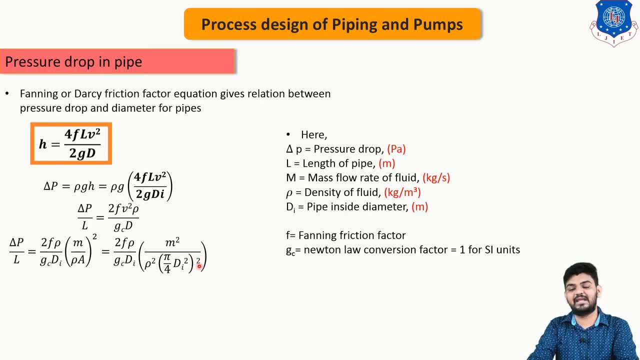 as pi by 4, D, I square and entire bracket has a square, since we were having area square. So if I give simplification to entire this equation, then I will. then then we can cancel out one density from here and we will ultimately have equation which look like this: 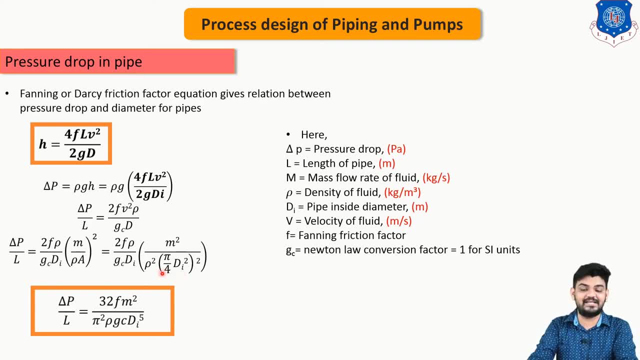 So, as you can see here, this 4 will be square, that is, 16.. 16 will be come to the numerator of the equation and it will be multiplied by 2. Hence we have here 32.. Then we have common friction factor as F. Then we have cancelled out our rho with this. 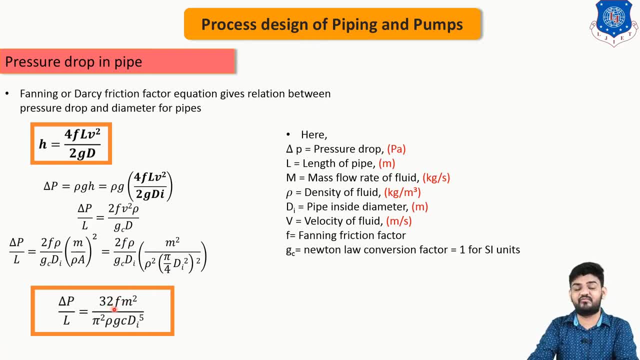 particular rho. So we have 32F M square which is being divided by pi square. rho g, C, D, I raise to pi. So this particular equation is again very important since it has been used to calculate pressure. So this particular equation is again very important since it has been used to calculate 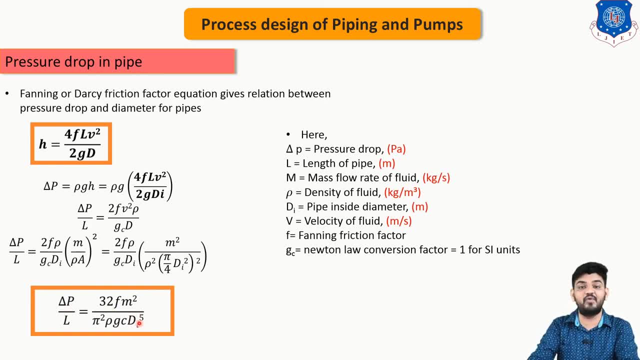 pressure. We know that this is the pressure drop for particular inside diameter of our pipe, So this particular equation is being used to design our pipes. Well, this equation is very important as there are always some sum based on this particular formula, And we are going to use this formula for further derimation as well. 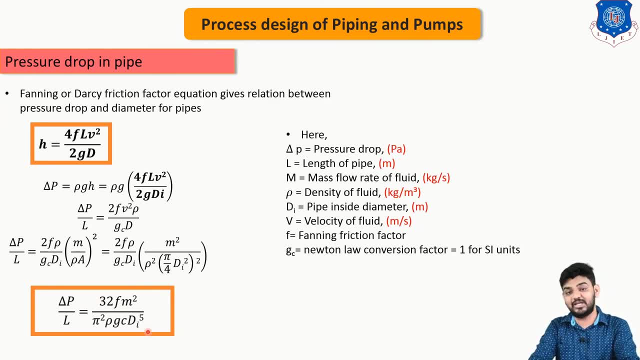 We are going to discuss one example based on this particular formula in the next video. Now lets us understand each and every term one by one Here. the delta P is nothing but your pressure drop and its unit should be in the pascal right. So here you have to remember always that the pressure in this particular formula is in the pascal right and that this is the air, which means length of our pipe. it should be in the meters. 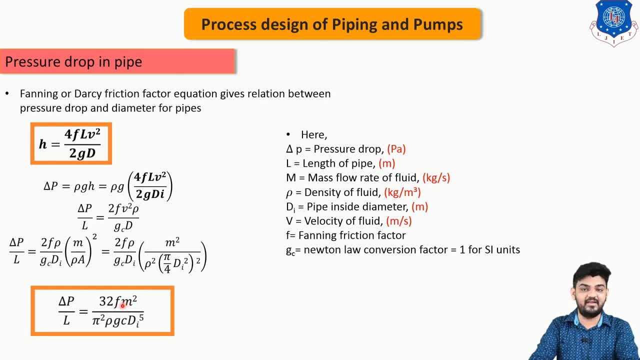 Then we have tidal friction factor, which do not have any units. This is the mass flow rate, which has the unit of kg per second. Then we have pi. then we have rho, which is the density of our fluid. that means kg per meter cube is its unit. 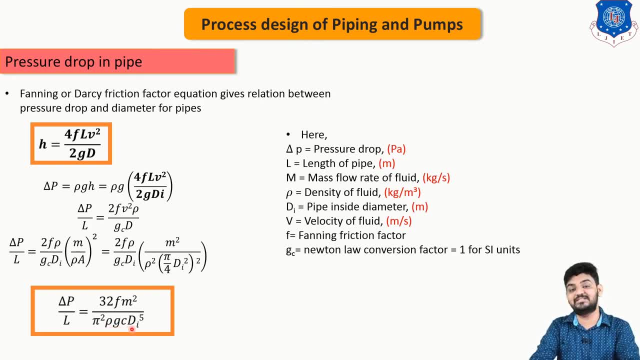 Then we have gc, which is again unit less, and lastly, we have inside diameter of our pipe as dn with the unit of meter right. So this particular formula is very important for calculation the pressure drop inside our pipe, right. So the main thing in this formula is this fan encryption factor and inside diameter right. 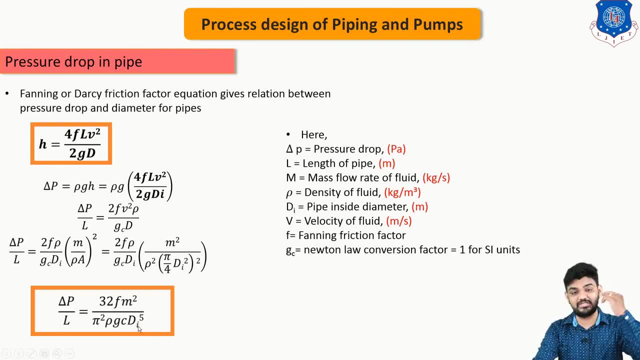 So To calculate inside diameter we have to assume velocity at the first step. So the first step will be assuming velocity and based on that velocity we have to find diameter, and then later that particular diameter is being used in this formula to calculate pressure drop. 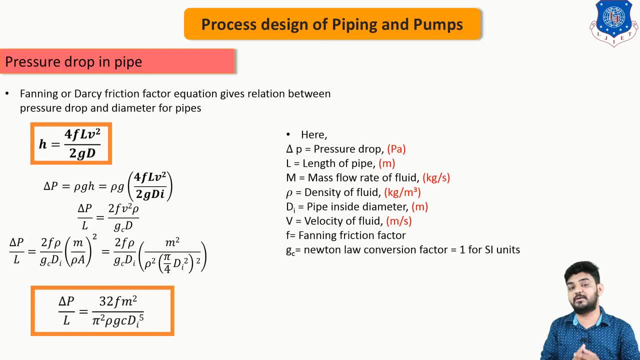 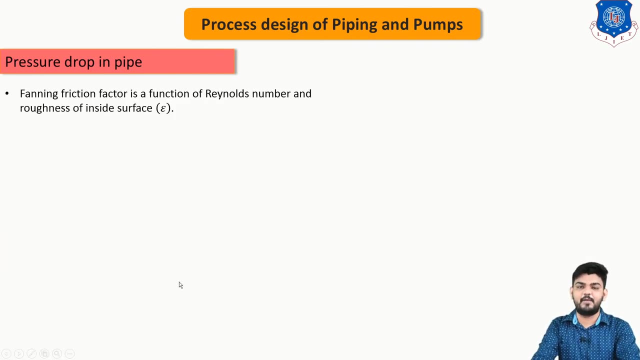 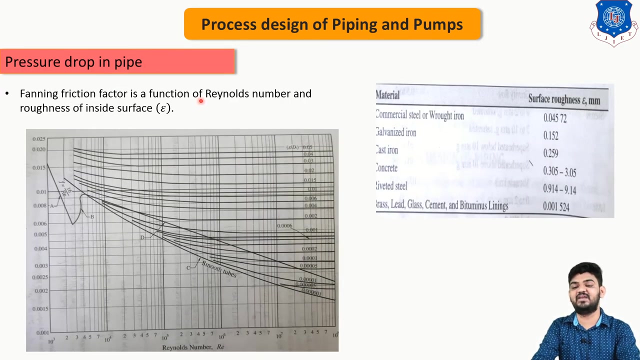 This sequence will be understood very easily when you will solve some ways, some based on this particular formula. Now the second most important thing from this formula is the fan encryption factor. How do we can find this fan encryption factor Right? In some example this friction factor is used to give. but in case, if this friction factor is not given, then you can see here the fan encryption factor is basically function of the Reynolds number and the roughness of inside surface. 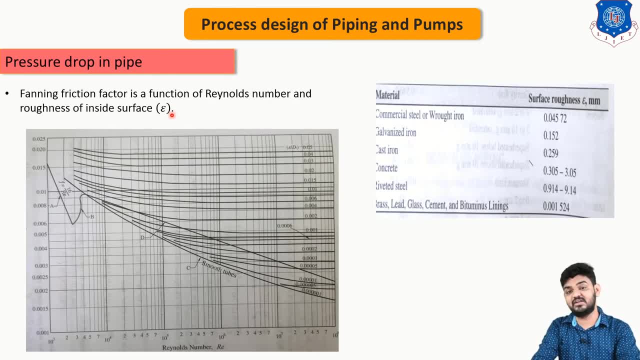 That is our epsilon. So we can find the fan encryption factor based on Reynolds number and epsilon. So here are some chart which basically reflect epsilon for different material, As you can see, As you can see here common steel has the epsilon is equal to 0.04572 mL.